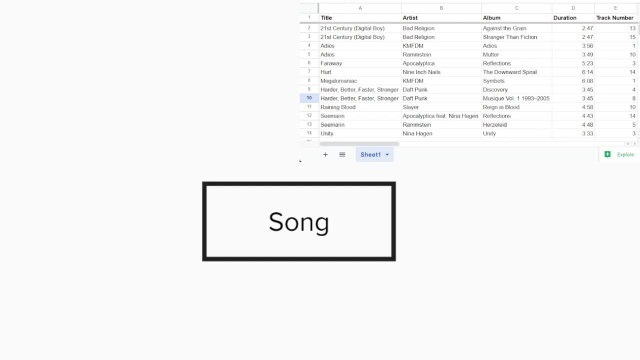 song is an entity type. The list in the corner contains various entity instances. This collection is an entity set, though there are, of course, many more instances of songs that we could include. Entities can possess various entities. Some attributes of a song could be its title, artist, album track number and duration. 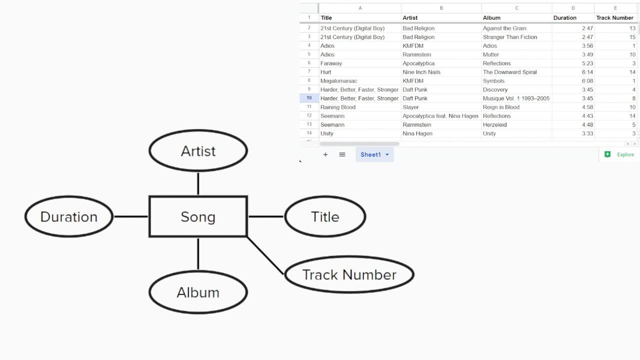 Whether or not a particular type of data is represented as an attribute rather than an entity of its own depends on the intended uses of the model. Some of these attributes will be depicted as entities later in the video. Here the attributes of song are depicted. 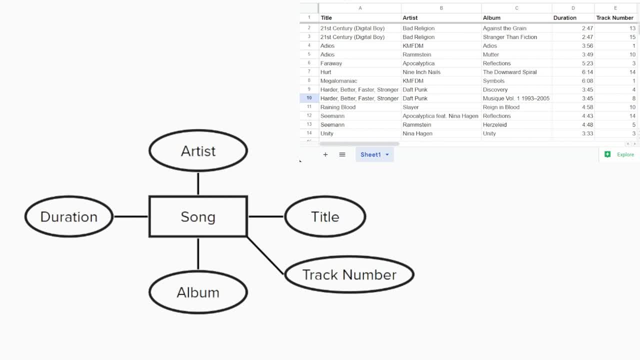 inside of ovals connected to the rectangular entity. Notice that for this data we have some repetition. The band Bad Religion released two different versions of a song called 21st Century Digital Boy on two different albums, And this entity set also contains two different songs with the title Adios, but by different. 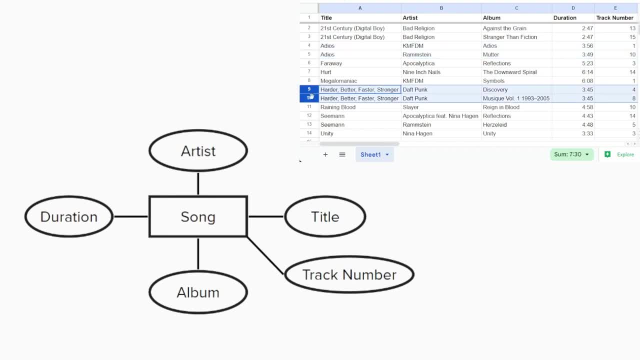 artists. The song Harder, Better, Faster, Stronger by Daft Punk is on the album Discovery, but that exact same recording is also on the Anthology album Musique Vol 1 1993-2005.. Another unusual case is the song Zeeman by Rammstein, originally but later covered by. 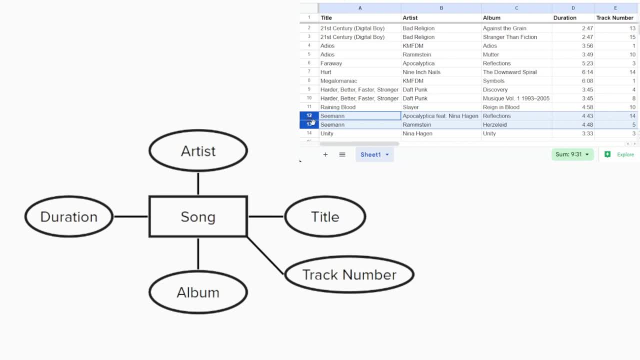 Apocalyptica. However, Apocalyptica's version of the song also features Nina Hagen as a guest artist. Does this mean that songs should have multiple artists? We could model the potential for multiple artists by drawing a double oval around the. 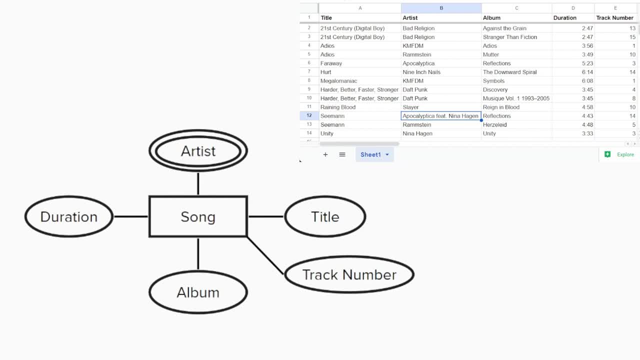 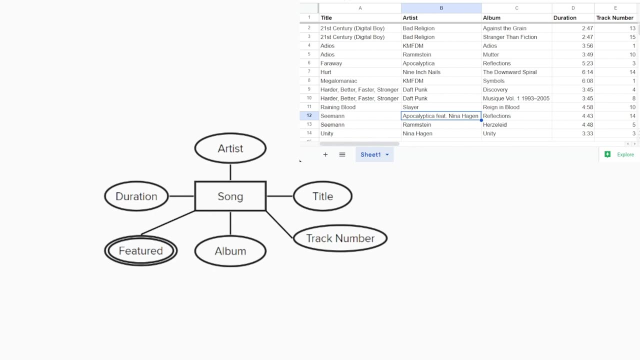 artist attribute like so. However, you could also argue that there is really only one artist and then a separate featured artist or possibly several featured artists. So let's separate out the featured attribute with a double oval on our diagram. like so We can also specify: 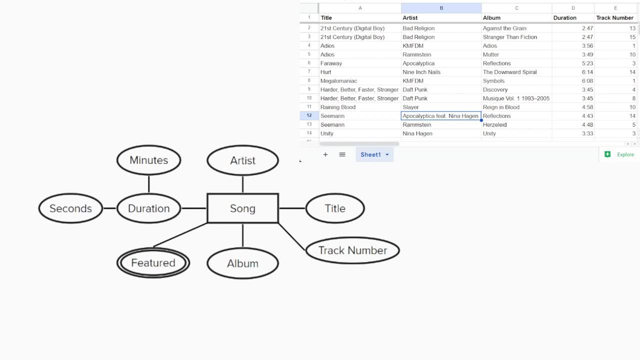 composite attributes, if we like. For example, the duration could be represented as a composite of minutes and seconds, in which case it would look like this. However, I'll return it to its previous form for the remainder of the video. Another example of a composite attribute could be a date that is broken up into day, month. 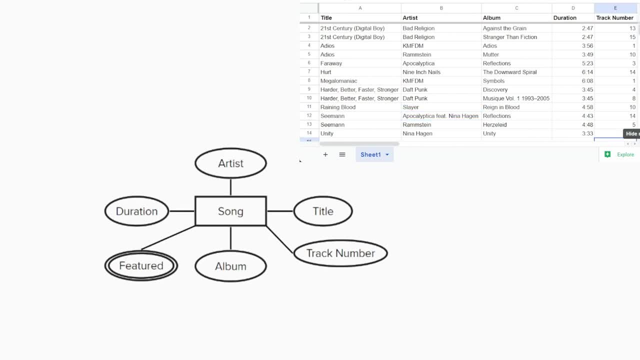 and year. Notice that with the repetition it can be difficult to identify an individual entity. Songs are not uniquely identified by their title Or even by the combination of their title and artist, since the band Bad Religion released two different versions of the same song on different albums. 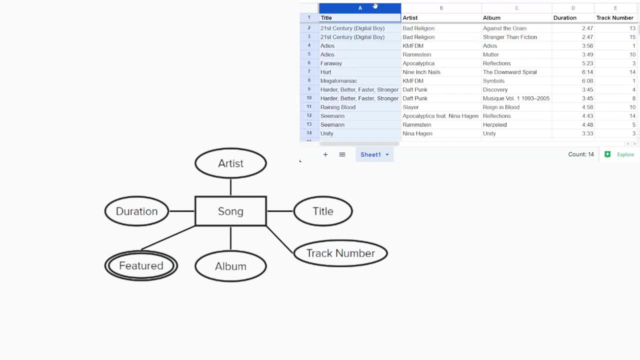 For this data at least, it looks like- the combination of title, artist and album can uniquely identify each song. The combination of title, artist and album is known as a super key because it uniquely identifies the instance. If we were to add duration and track number, then that set would also be a super key. but 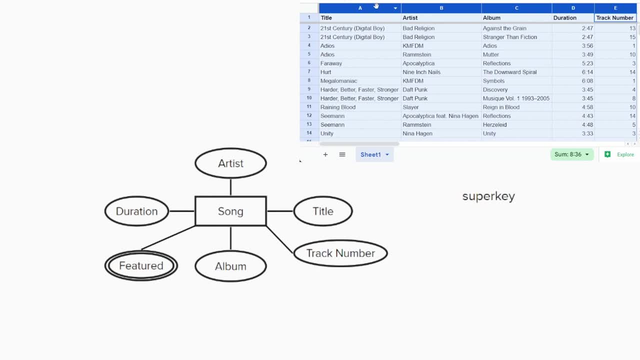 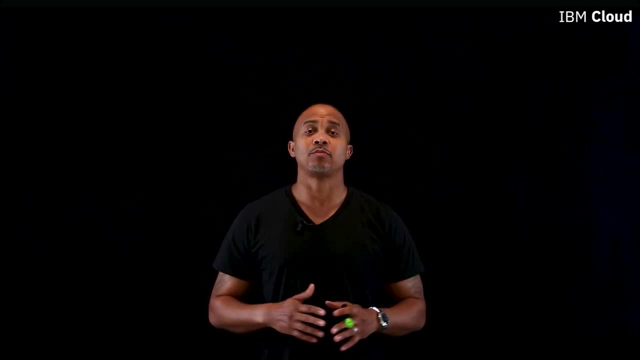 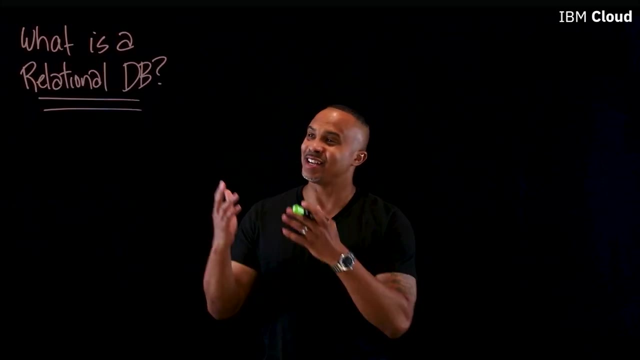 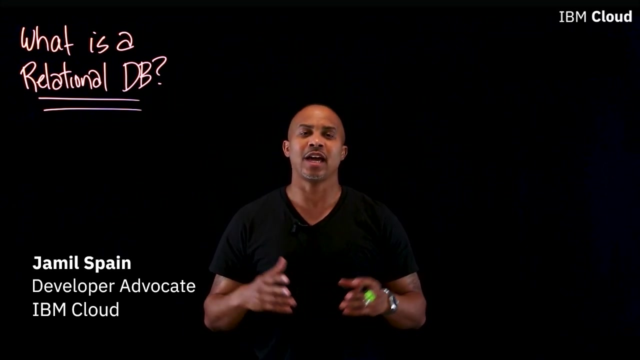 I've got a pop quiz for you. What database system has been around for almost 50 years? I guess you can guess it by the topic of this video: It's a relational database. Hello, my name is Jamil Spain developer advocate with the IBM Cloud and brand technical specialist. 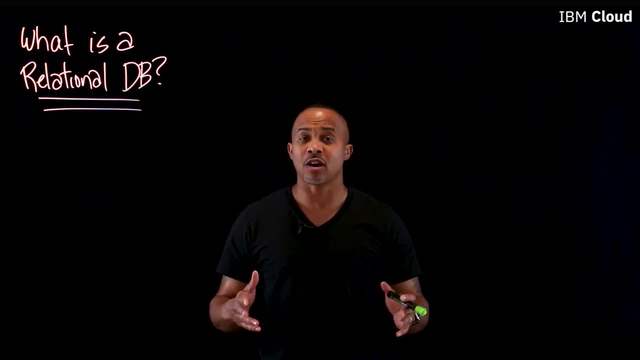 in the US financial services market. In today's talk we're going to dive a little bit into relational databases. I'm going to get into some of the characteristics of the database model and also some benefits that it provides for you when making your decision that you want to use. 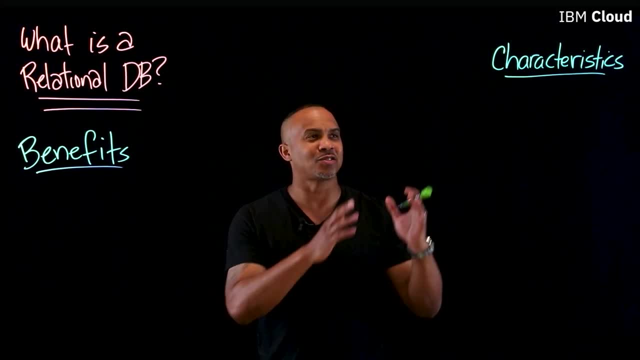 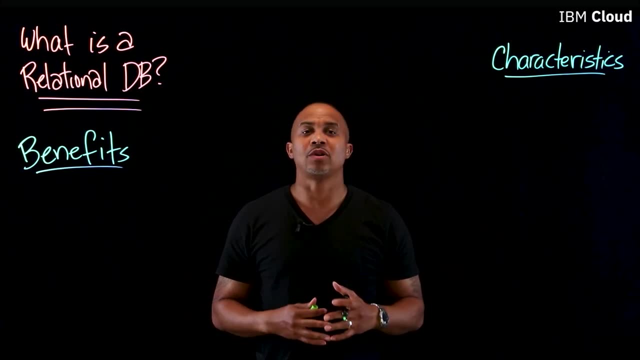 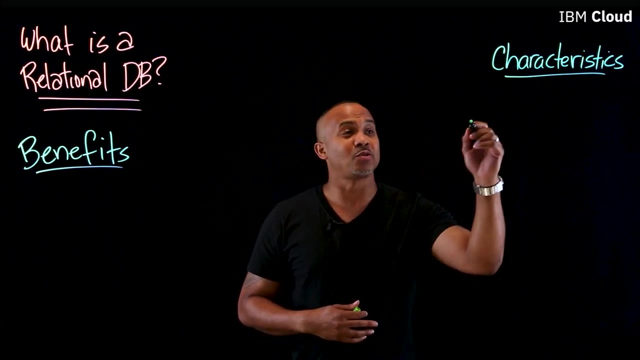 this for your next project. To get started, let's talk about the structure of a relational database system. It's going to pretty much map out your data points and bring out the relationships in that And the way that it accomplishes that is through the first thing. is making tables. So the first thing is making tables, And the way that it accomplishes that is through the first thing is making tables. So the first thing is making tables, And the way that it accomplishes that is through the first thing is making tables. So the first thing is making tables.